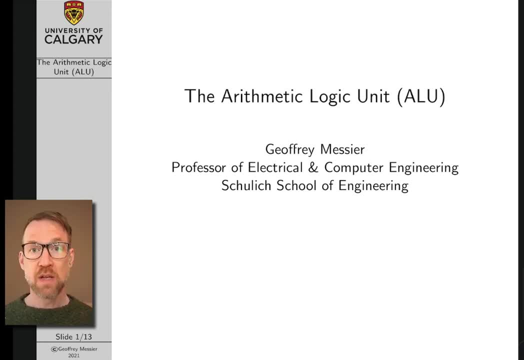 our microarchitecture and start talking about how we design digital structures to implement some of these number representations and mathematical operations And we, as you know, as this sort of the theme for this course, we are going to implement kind of a subset of the full. 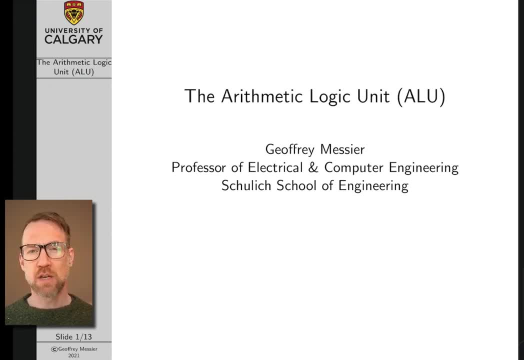 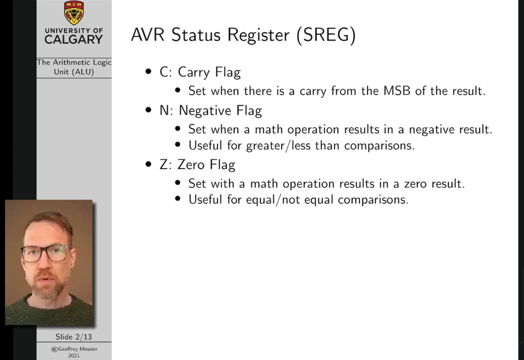 functionality that you could find on a typical AVR microarchitecture, But what we're going to talk about, I believe, is representative enough to give you a good idea about how an ALU is designed. Now, to start off, the AVR microcontroller has something that's known as a status register, or 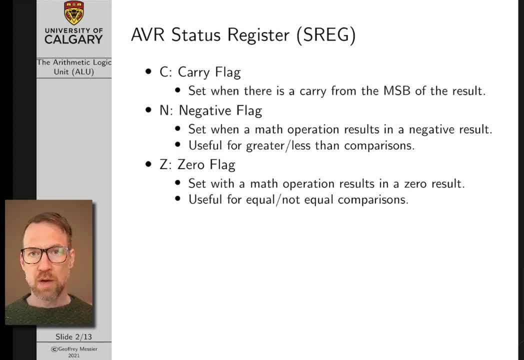 short, And the status register is a control configuration register, just an area in memory that contains a number of binary flags, So it's just an 8-bit register, but each bit represents a binary flag that, and most of them, are the result of performing a mathematical operation. 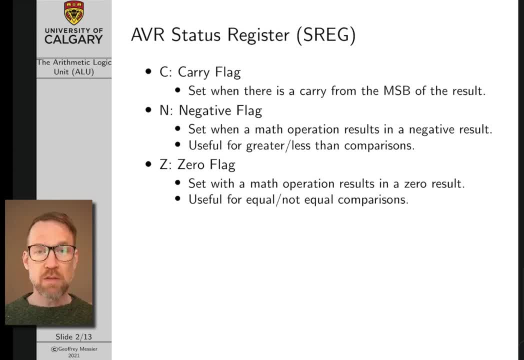 on two 8-bit numbers And there are a bunch of these flags, but we're just going to talk about a subset of them And we're going to see how we implement these flags within our ALU design. So the first flag is the carry flag And the carry flag is set when there is a carry from the most significant bit of 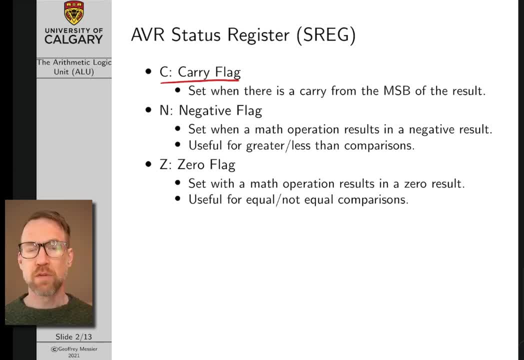 the of an addition result. So when you're adding two numbers together in your ALU, if they're, if the carry out bit from the most significant bit is addition is equal to one, then, uh, the carry flag is set. 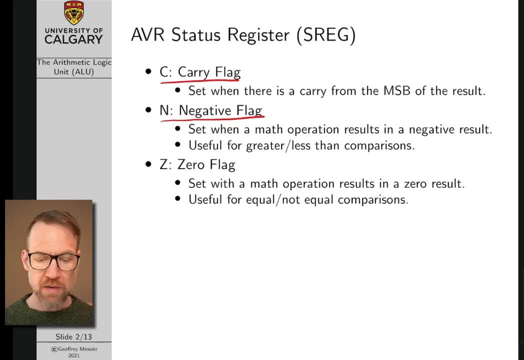 There's also a flag called the N flag or negative flag. This flag is set if the result of an ALU operation is negative, And typically this occurs when you're subtracting two numbers, and this is useful for not only knowing what happened with uh a subtraction, but also for Boolean tests. 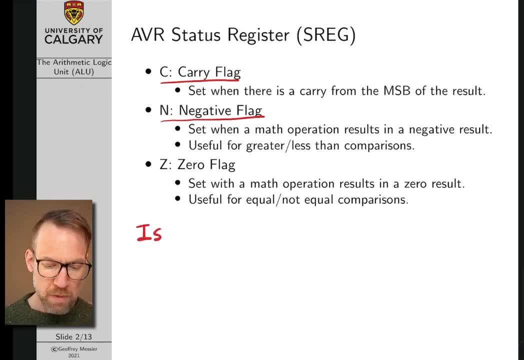 So, for example, we might want to test, you know, is a number a less than a certain number b? right, You can think of a lot of cases in a program where we're testing for a less than condition. The way we implement this in the AVR microarchitecture is: 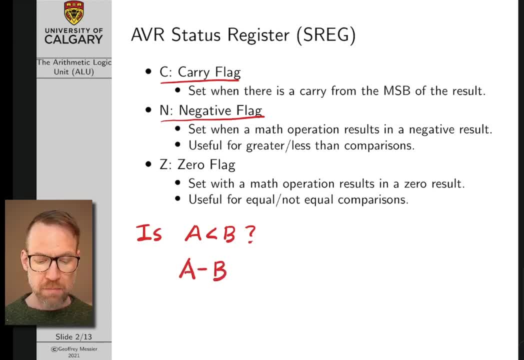 we perform a subtraction operation- a less than b- If the negative flag is equal to 0, That means that the and if a and b are two positive numbers. if n is less than zero, or sorry, if n is equal to zero, then we know the result of our subtraction was positive. 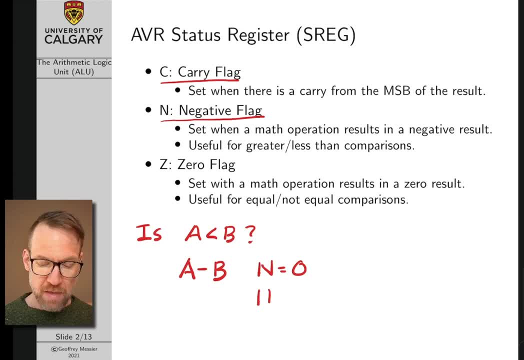 and a is less than b. If n is equal to one, then a was greater than or equal to b. So n is equal to zero indicates that a is less than b, n equal to one indicates that a is actually greater than or equal to b. Finally, the zero flag is set when a mathematical operation results. 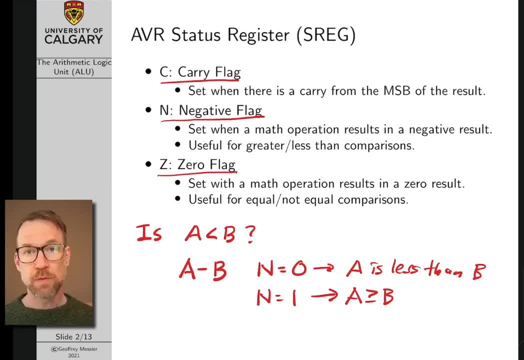 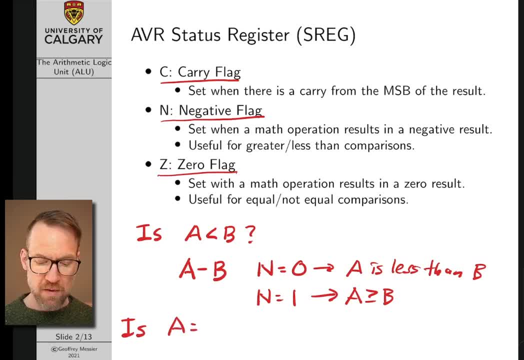 if we want to say, if we want to test, is a equal to b? what we do is we just subtract those two numbers And if the zero flag is equal to one, a equals b. If the zero flag is equal to zero, 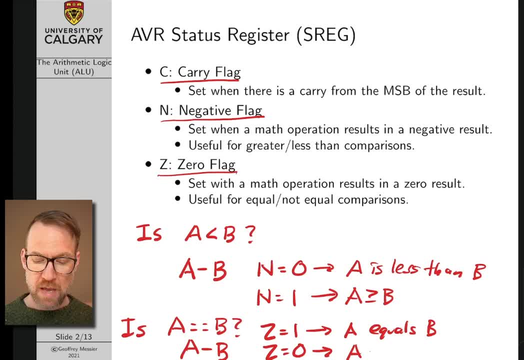 we hit, we got a non-zero result from our operation and a is not equal to b. So these three flags are generated within the ALU and, like I said, as we implement our ALU design, we'll see how we design our ALU, not only to generate a mathematical result, but 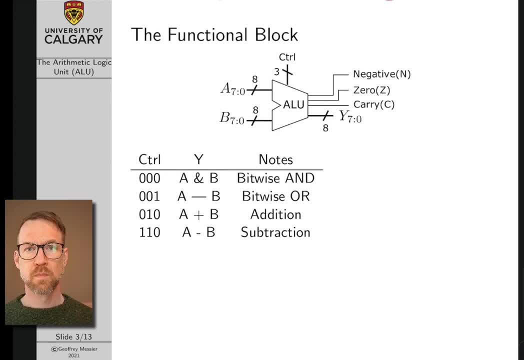 also to generate these flags as well. So in previous lectures, when we've drawn our micro architecture, we've seen that our micro architecture consists of a number of functional blocks. So we had a functional block that represented the data memory, a functional block that represented the 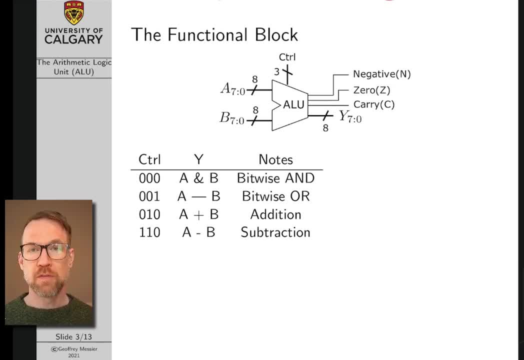 instruction memory. This is the functional block that represents the ALU. ALUs are often represented by this distinct semi-triangular shape and in our case our ALU has two inputs: an 8-bit number a and an 8-bit number b. So we've seen that our micro architecture consists of a number of functional 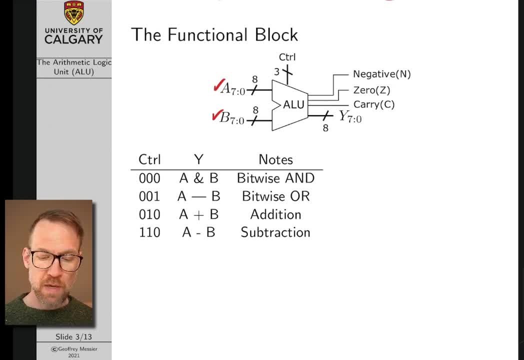 blocks: an 8-bit number a and an 8-bit number b, an output, an 8-bit output y and three single bit digital outputs that represent the negative flag, the zero flag and the carry flag. We also have a three-bit control bus and we change the value of the three-bit control bus to 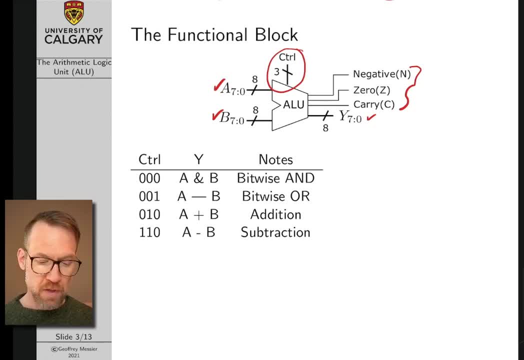 change the mathematical operation performed by the ALU. Again, we're only going to focus on a subset of the actual number of mathematical operations that the ABR ALU is actually capable of and for the purposes of this lecture, we're going to focus on the bitwise AND operation, which is performed when our three-bit control bus is equal to zero- zero. 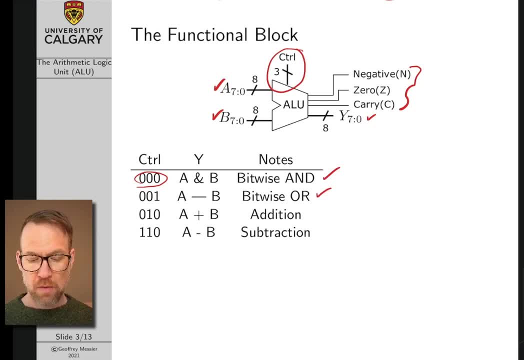 zero, The bitwise OR operation. we have an addition operation and a subtraction operation, And the number representation we're going to be using will be eight. bit twos complement Now one of the blocks, one of the the basic digital logic blocks that we're going to use to implement. 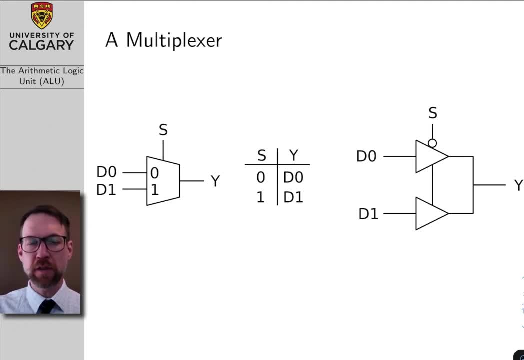 our ALU is a multiplexer, and basically a multiplexer allows us to choose from several possible inputs and choose one of those inputs and connect it to the output of our block. And so the simplest possible multiplexer is shown right here, where we have two single line inputs, d0 and d1. so 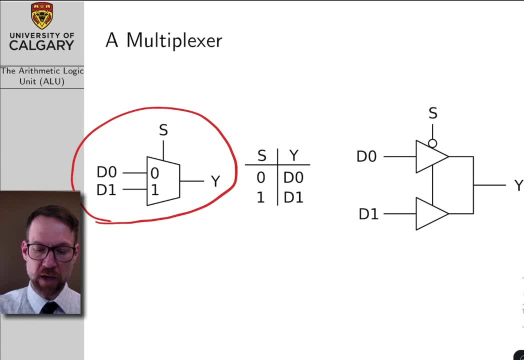 these are just single logic lines. We have an output y and we have a selector line, s, and the truth table for the multiplexer is right here. so if s is equal to zero, y is equal to whatever logic value is on input d0.. And if s is equal to one, y is equal to whatever logic value is on input d1.. So we can just choose. 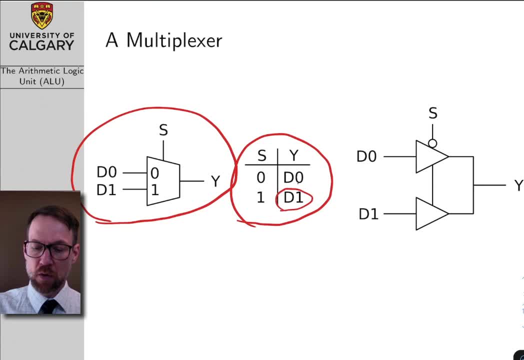 from one input and direct it through to the output. There are a few different ways to implement multiplexers. One way is to use tri-state buffers, So we have a series of tri-state buffers. This little circle of course indicates the NOT operation or inversion, And we connect. 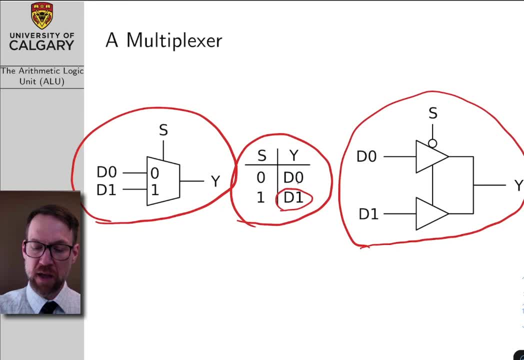 our tri-state buffers to the input d1.. So we have a series of tri-state buffers- This little circle of course indicates the NOT operation or inversion- And we connect our tri-state buffers to the input d1.. And this boolean is linked to a common output, y. And when s is equal to zero, this little inversion. 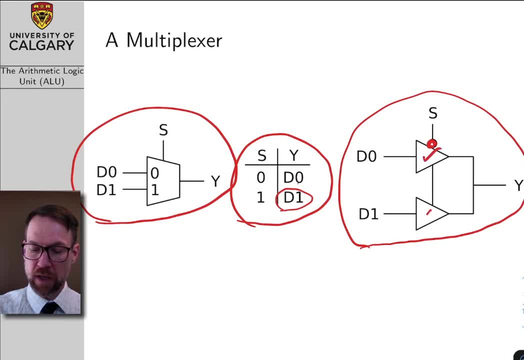 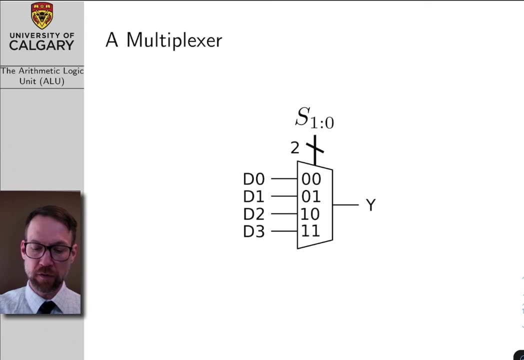 bubble will enable the first tri-state buffer and disable the second one, And when s is equal to one, it's the other way around. You can, of course, have more than one input in a multiplexer, So this is an example of a four input multiplexer, where 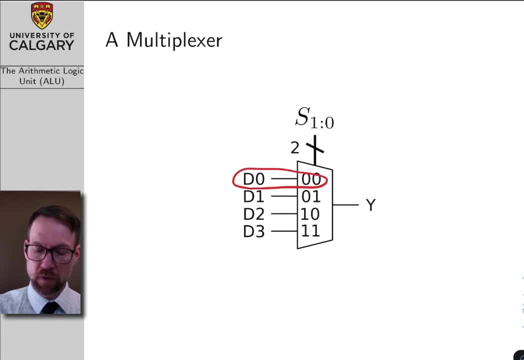 selects d0, 0. 1 selects d1, 0. 1. 0 selects d2, 1, 1 selects d3, and whichever input is selected, that's what you can think of it as sort of being connected to the, the output y. So if we have 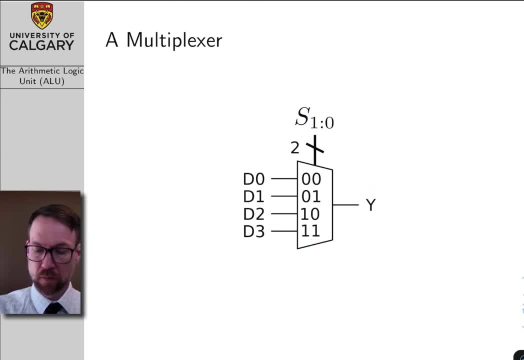 our input equal to- or- sorry, if we have our selector, our two-bit selector lines, equal to 0, 1. for example, y is going to be equal to d1.. Now what we're going to see in the upcoming slides are multiplexers that don't just have single line inputs but take buses as inputs. So 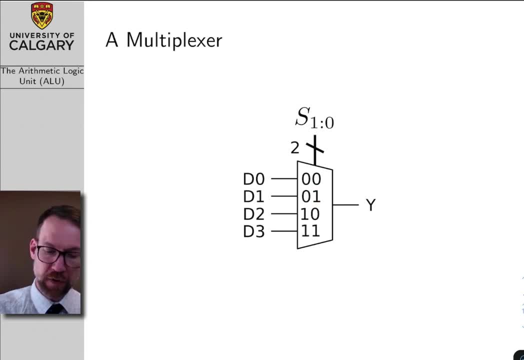 for example, you'll see a multiplexer where you know this might be an 8-bit bus. each of these inputs might be 8 bits, and then the output would be 8 bits as well, And it works basically exactly the same as the single line multiplexers. So, for example, if our selector bus was equal to 1, 1 y would be equal. 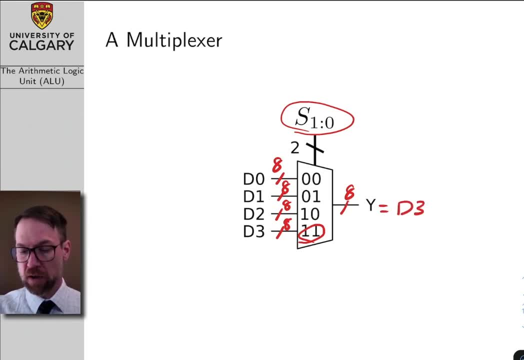 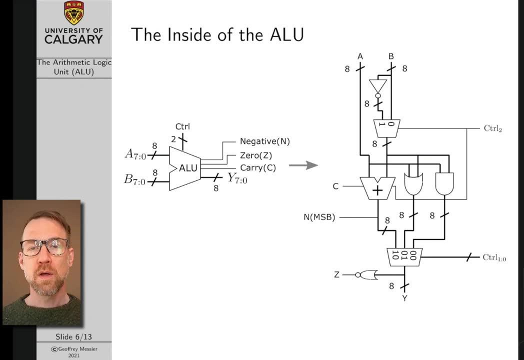 to d3, but all eight parallel lines of y would be equal to the eight parallel lines of d3. all right, now we're going to zoom inside our ALU block and see how it's actually implemented using basic digital logic gates, and so this is the high-level ALU picture that we introduced at 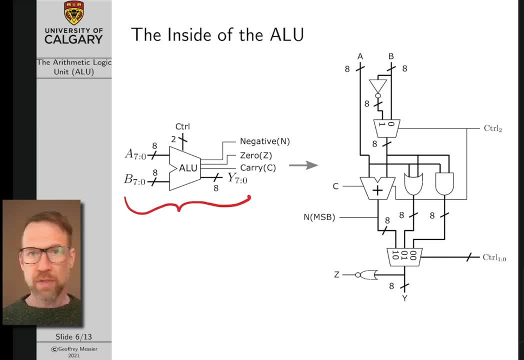 the start of the lecture and if we zoom in, if we pull the the top off the ALU. this is what we find now just to sort of orient orient everything. we have our two 8-bit inputs, a and b. we have an inverter block that does a bitwise inversion on each of the 8 bits. we have a multiplexer block. 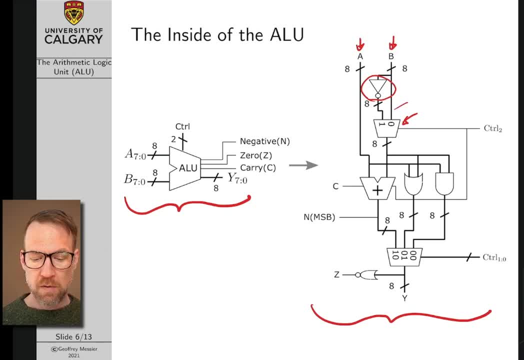 that will choose the right hand 8-bit bus input or the left hand 8-bit bus input, depending on the whether this single control bit is equal to 0 or 1. we have an AND gate that performs a bitwise, AND on the two 8-bit inputs we have an OR gate that performs a bitwise, OR on the two 8-bit inputs we. 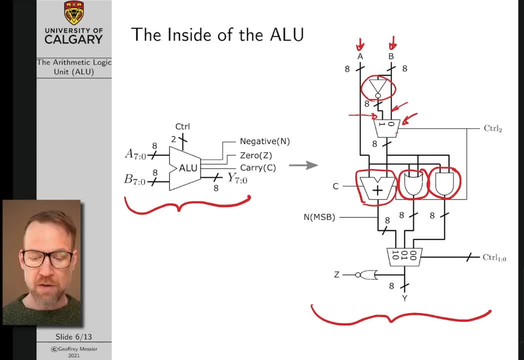 have an adder block that performs binary addition on the two 8-bit inputs. we have a multiplexer block that selects from three possible 8-bit outputs depending on the value of a 2-bit control bus. we have a NOR block that calculates a NOR operation on all of the 8 bits and produces a 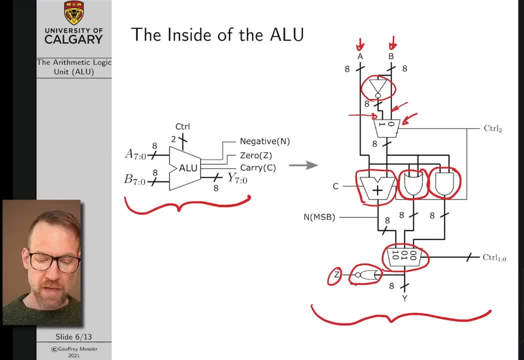 a single bit output. this is the zero flag. the carry flag comes out from the 8-bit adder and the negative flag is just the most significant bit coming out of the 8-bit add result. so the remember we have. sorry, this should be a 3-bit control bus. this is the most significant. 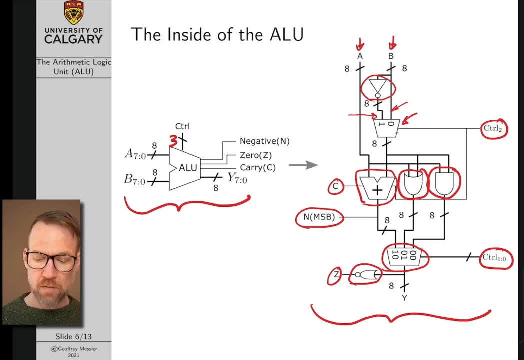 bit of the control bus, and this is- these are the two least significant bits of the control bus, and so, basically, what we're going to do, if I kind of wipe away all of this scribbling, this digital structure is able to perform the bitwise AND operation, the bitwise OR operation. 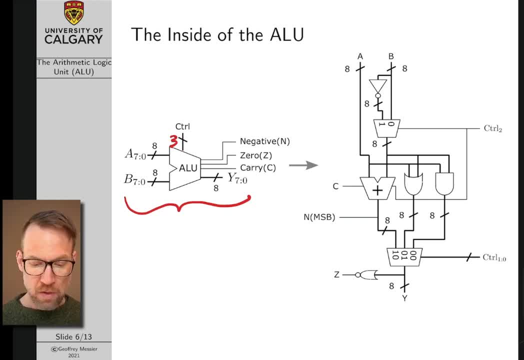 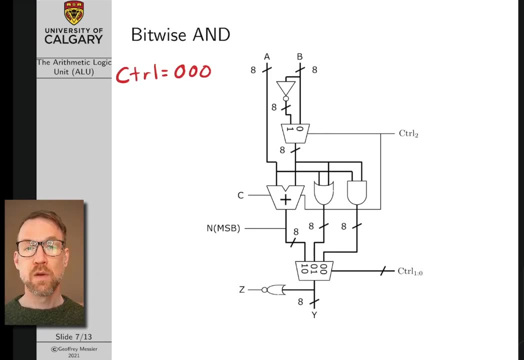 addition and subtraction, and what I'm going to do in the next few slides is basically step through each one of those operations and show which part of this digital structure is activated to perform each one of those operations. okay, so let's start with the bitwise AND operation, which is one of the easier ones. 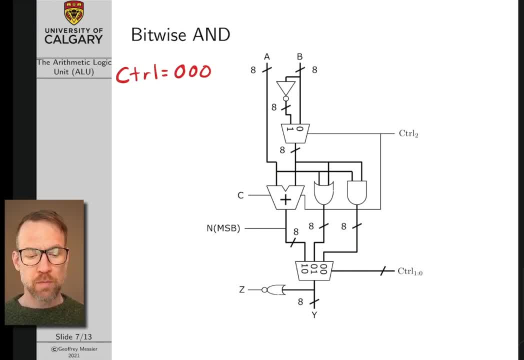 in order to perform bitwise. AND the 3-bit control bus is equal to 0, 0, 0 for our ALU. so that means our most significant bit is 0, so this control line is 0, and our least two significant bits are also both 0, so we have 0, 0 here. now we're going to perform the bitwise AND operation. 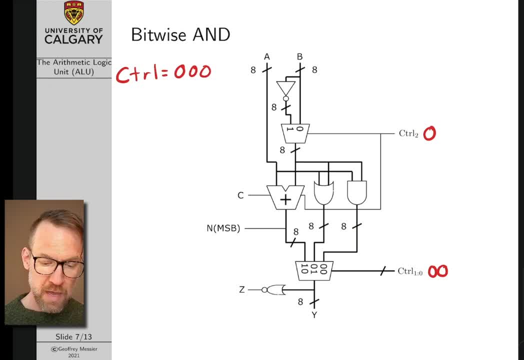 between our two inputs, and so our first input, a, feeds down here and actually is connected to three of our logic blocks: the adder, the or and the and b feeds into a multiplexer, but because our control line is zero, it's the right hand bus that gets selected, and this bus or this 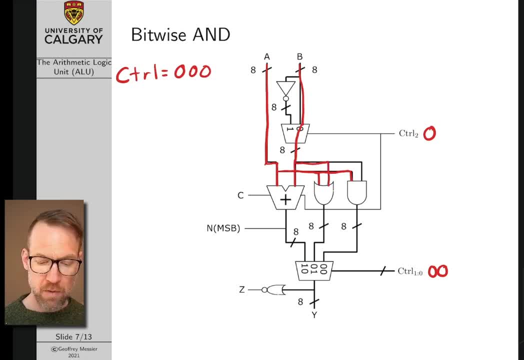 bus goes into the other input for our AND, OR and adder blocks. so we've got all three of our or the, the AND block, the OR block, the adder block, the OR block and the AND block are all operating here, but we're only going to take the result of the AND operation and the 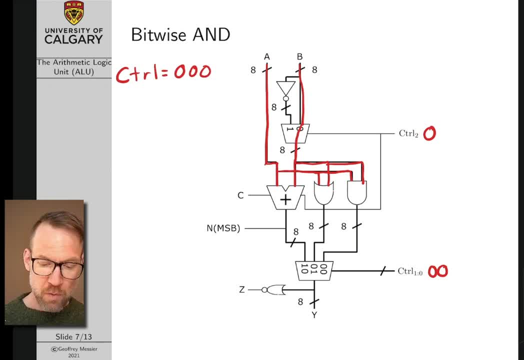 way we do that is by this bottom multiplexer. so all three of these blocks are generating results, but the only output we're going to take- because our control line is equal to 0, 0- we're going to take the result of the AND block and that goes out and appears at the Y output. so you'll see like: 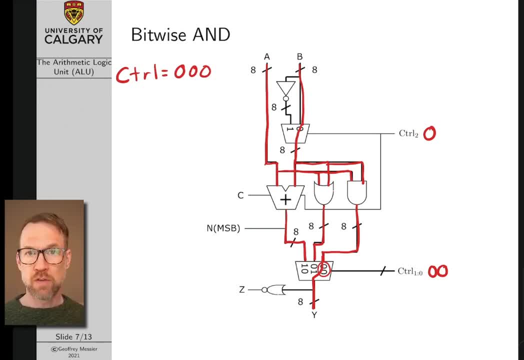 we've got all the hardware for all the operations. and the hardware, because it's combinational logic, is just firing away and doing its calculations anyways, but we use the multiplexers to pick the results that we want. now the bitwise OR operation works in a very similar way. so to do bitwise OR, our 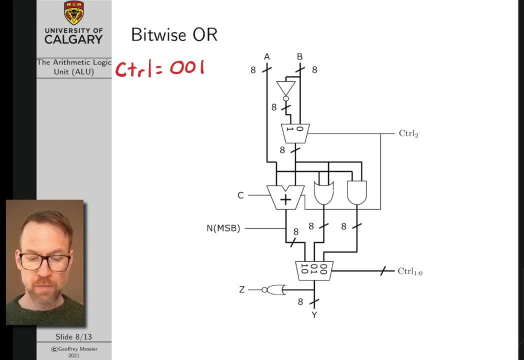 control bus is equal to 0, 0- 1, so that means we have 0 up here and 0, 1 down here. our A input feeds into again all three of our blocks. our B input, because control 2 is 0, 0 is selected without inversion. 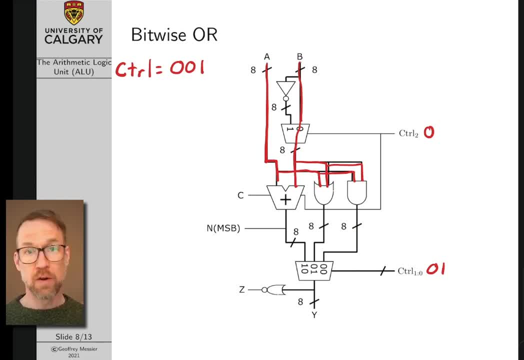 all three of our. so the AND, the OR and the adder are all again producing results, but it's the OR result that we select, because our control line now is equal to 0, 1, so OR appears at the Y output. so the addition operation again is is very similar. so we have our A bus. 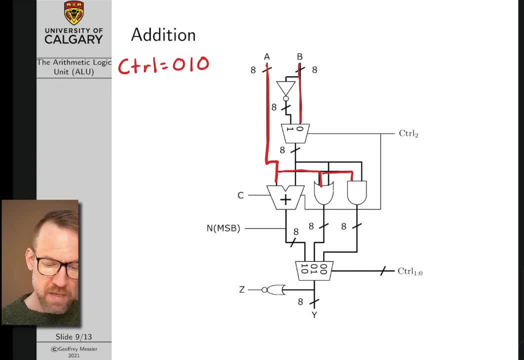 going into all three of our logic blocks. B, because our most significant control bit is equal to 0, is passed through the multiplexer without inversion. and all three of our blocks, the, the AND, the OR the adder. they perform their operations, except this time it's the adder that we select, because 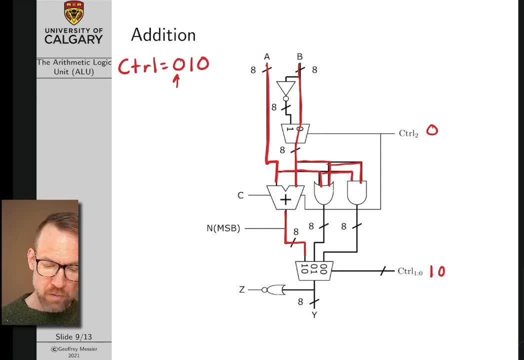 our lower control lines are equal to 1: 0, and so it's the result of the adder that appears at the output of the Y. the C flag is the carry out bit of the most significant bit. addition operation. the addition operation for the most significant bit. 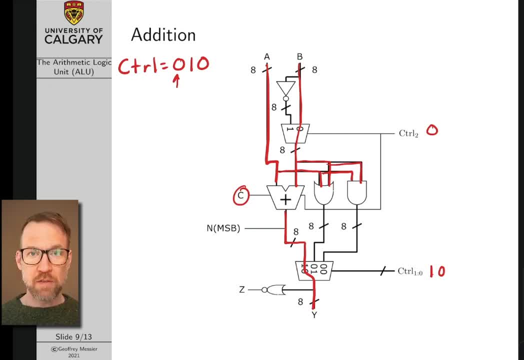 and to understand that more fully, we need to investigate the design of this adder block a little bit more carefully. so what we're going to do is we're going to zoom inside this adder block and see exactly how it's implemented, as you're going to see. 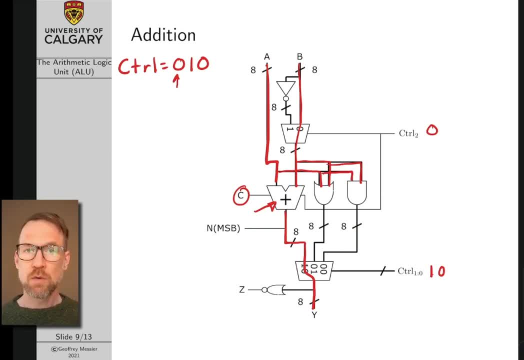 it's basically what we call, or what I'm going to present to you is what's known as a ripple adder, where our two eight or the addition of our two eight bit numbers is actually made up of eight one bit addition operations that are all sort of strung together. 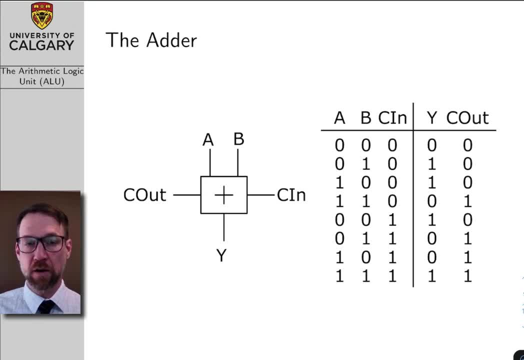 so the basic building block of our adder, our 32-bit adder, is this, which is our one bit adder, so I guess maybe I should have said one bit adder. this adder adds two bits together, so A and B are the two input bits that we're adding together. these are single logic lines because we're only 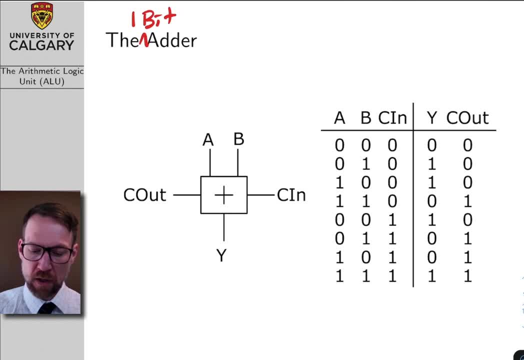 adding one. we're only adding single bit values. this is the carry output line and this is the carry input line. you can think of carry input as sort of a third input bit. so really we're adding three bits together. we're adding A, the the single bit adder to output. Y is equal to A plus B. 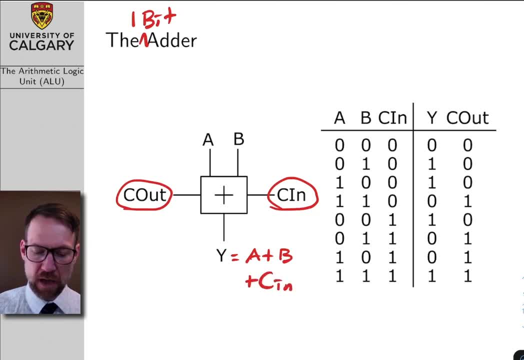 plus C in, with C out as being the output carry bit. and so this is the the logic table for our one bit adder. if all of our inputs are zero, the summation, the sum value Y, is equal to zero and the carry output bit is equal to zero. if. 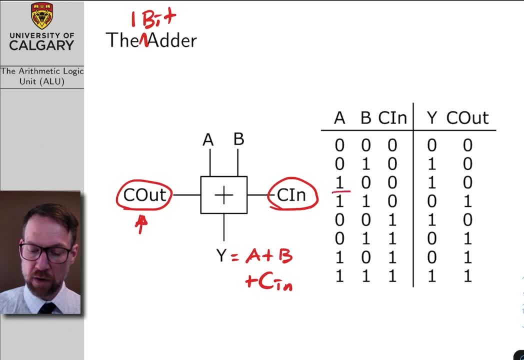 we have. if only one of our input bits is equal to one, then we have Y equal to one and our carry output equal to zero. so this is just like adding up zero one zero, so this is equal to one and we don't carry anything. this is basically the same thing as down here. so if A and B are equal to zero, but our carry 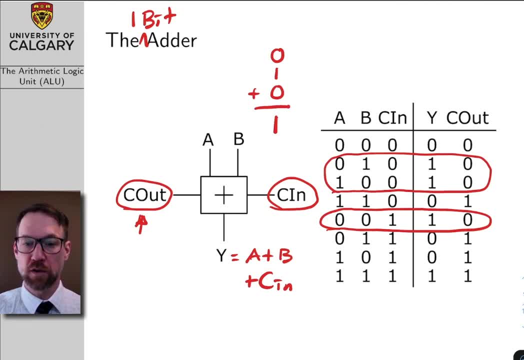 in input is equal to one, then it's just like adding one to two zeros. if we have two ones being added together, either if A and B are both equal to one, or if either A or B are equal to one and C in is equal to one. right here. 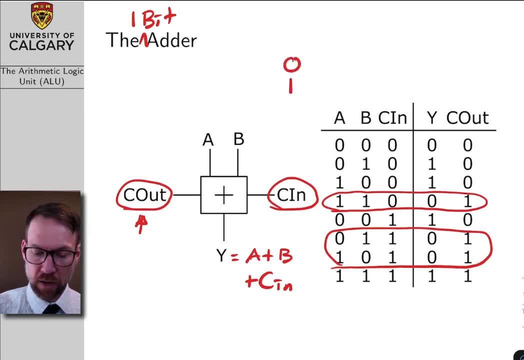 we have the situation where we're adding zero, one and one, so when we add that together we get zero, but then we have a one bit that we carry on to the next column of addition, so our C out output line is equal to one in this case. and then, finally, the last situation is when we have 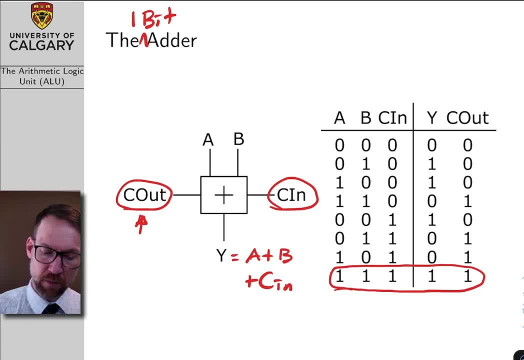 all three of our inputs equal to one, and so that corresponds to 2 plus 1, to 1 plus 1 plus one, so we get 1, so that's three. right, three is equal to one one, so we have one, and then we carrying the one there. so 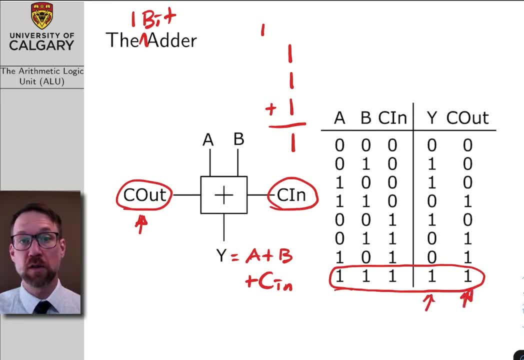 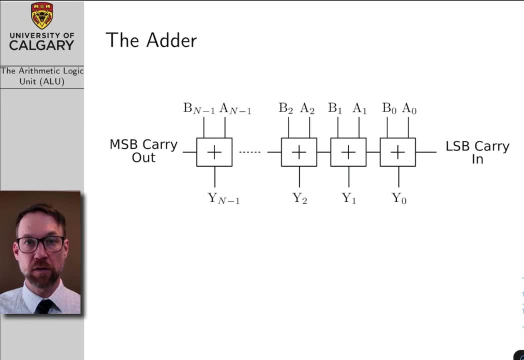 Y is equal to one and our carry output bit is equal to one, and so if we want to create an adder that takes, you know, 32 bit numbers in parallel and produces a 32 bit output, we basically just cascade together a whole bunch of these single bit adders. 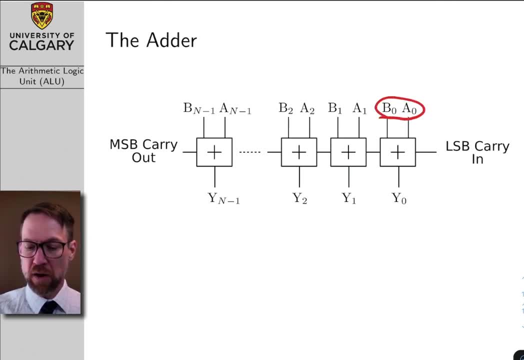 So B0 and A0 are the two least significant bits in our A and B 32-bit parallel arguments being added together. And this is the least significant bit of the output bus Y0.. Now you'll note that the carry output of our least significant bit is connected. 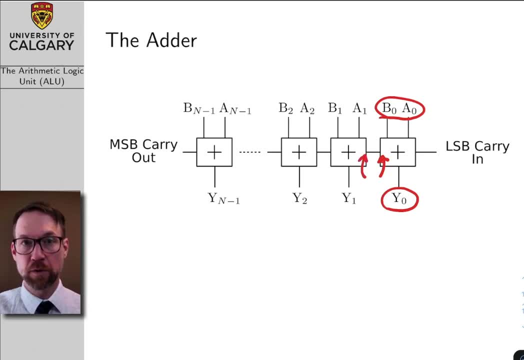 to the carry input of the next most significant bit, And that's just the way how binary addition works. So, for example, we've done a few. let's say we're adding two plus two binary, we add zero plus zero, which is zero. 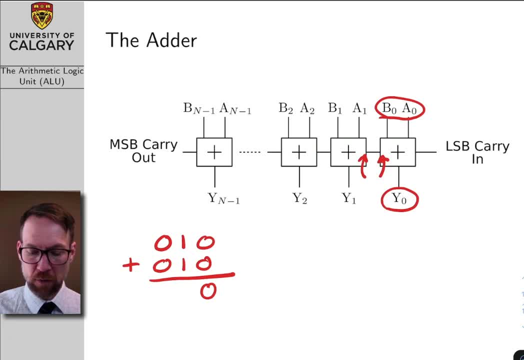 Now, normally if we have no carry bit, we don't write it, but in this case, really, the carry bit is equal to zero, And so we take the carry bit and we put it up there. Then we have zero plus one plus one. 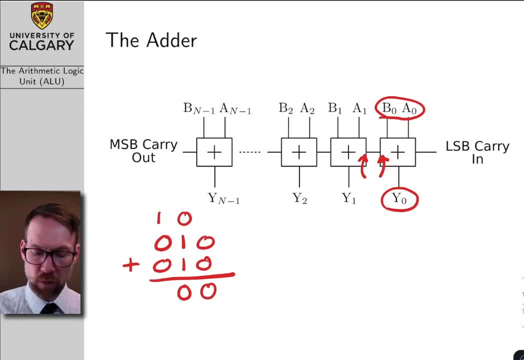 which is zero, with a carry bit of one. And then we have one plus zero, plus zero, which is one, with a carry bit of zero, and so on. So the carry output of the first column is the carry input of the second column, The carry output of the second column. 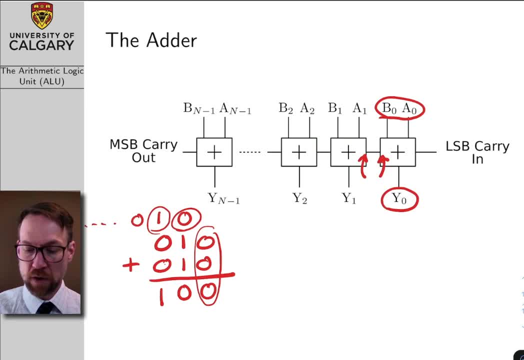 is the carry input of the third column, And so on, So you cascade all of these together And this, as you might imagine just from the way it's connected, this is what's known as a ripple adder And, for the case of the MIPS ALU that we're working on, 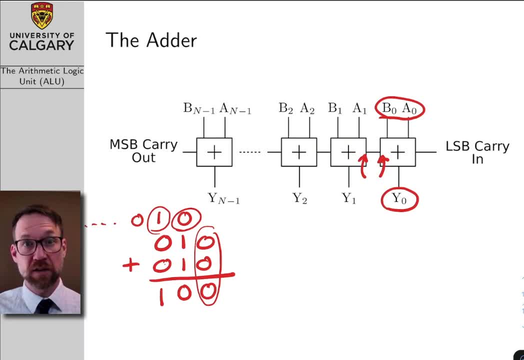 we would have 32 of these one bit adders connected in a cascade to implement the adder block that we showed a couple of slides ago, And you'll notice that the carry input for the least significant bit is still used as an input to our adder. 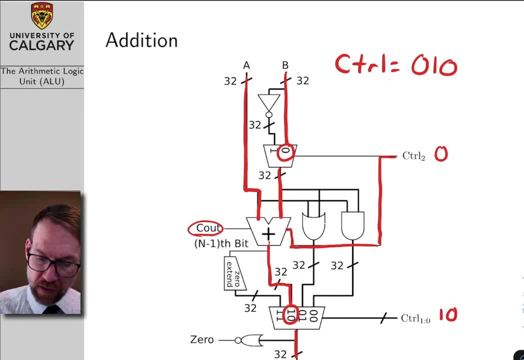 So this input here is the carry input for the least significant bit in our cascaded adder, And so when you look at this adder block you can just understand these as 32, single bit adders cascaded together, The carry in input for this big adder block. 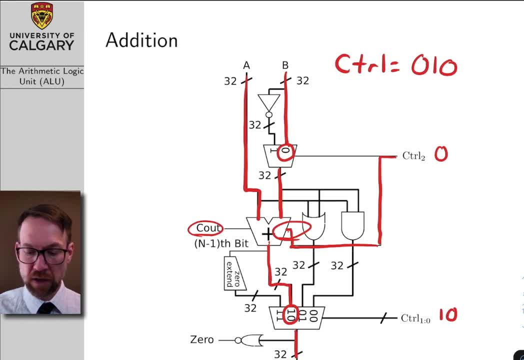 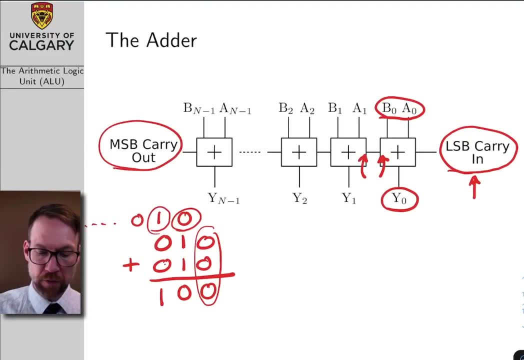 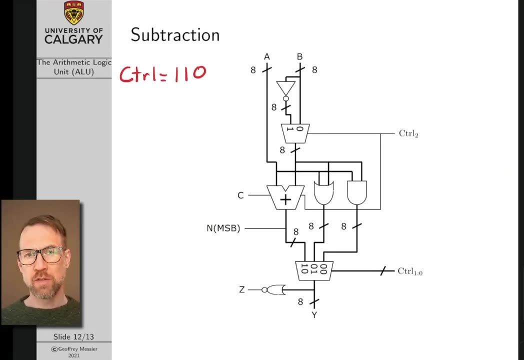 is connected to the carry in of the least significant bit, And this cout output is the carry out of the most significant bit. Now, finally, the subtraction operation is broadly the same as the other operations, but there's a few kind of subtle, interesting little tricks. 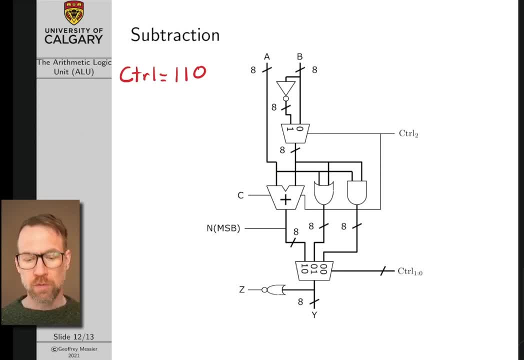 that we do to actually implement the subtraction operation. So the first thing you might've noticed is that we had a dedicated logic block for each of our first three operations, right So? and had an and block, or had an or block. addition, had an adder. 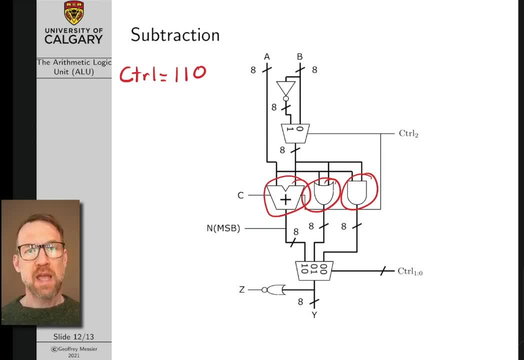 There's no fourth subtraction block And what we actually end up doing is we use the adder to implement subtraction, but we do this by inverting one of, or negating one of the input arguments. So the way that we implement a minus b. 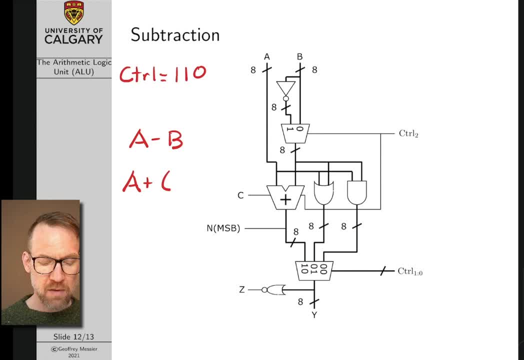 is actually by adding a with the negative value of b, And now we finally get to see what this inverter is. So we can see that the adder is for and also, interestingly, why we have a control line hitched up. 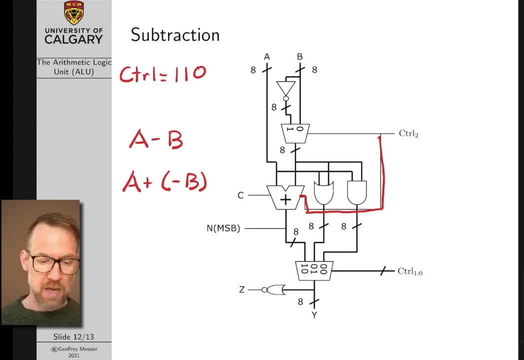 to the carry in input of the adder block. So I'll just erase some of this stuff here, So remember. so our A bus goes into the adder. as usual, Our control lines for subtraction are one one, zero. So down here at our lower multiplexer, 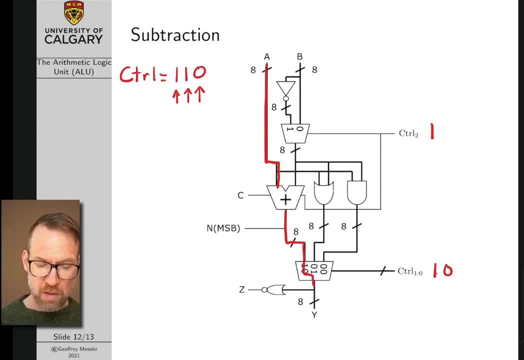 that means that we're just gonna take the output of the adder and feed it out onto y, So that looks exactly the same as addition. However, it's this control two line up here, being equal to one, that's actually going to take care of the negation. 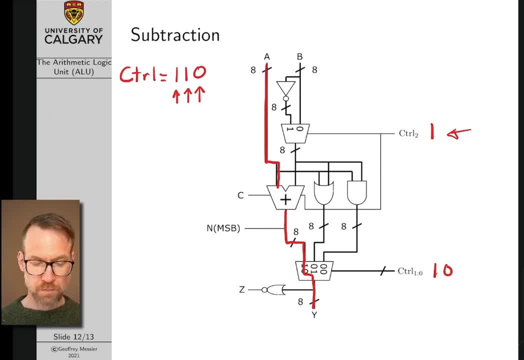 operation for the argument b. So remember that in order to negate a two's complement number, you don't just do a bitwise inversion. You do a bitwise inversion and then you add one, And so having this control line equal to one means that instead of selecting the non-inverted b input, 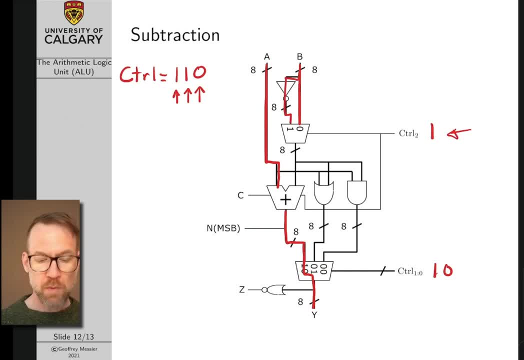 we take the bitwise inversion, the bitwise inverted version of it, and pass that through to our output. So at this point where I've drawn the arrow, we've done a bitwise inversion of b, but that is not quite the negative value of b, right? 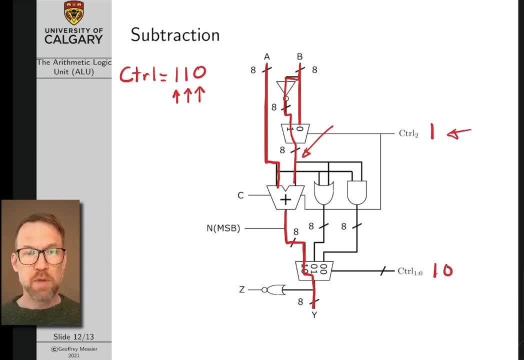 Because we still have to add one. Just doing a bitwise complement or a bitwise inversion of a number does not necessarily or does not equal its negative. in two's complement, We still have to add one. The way that we add one is by connecting the carry in line to this control. two: 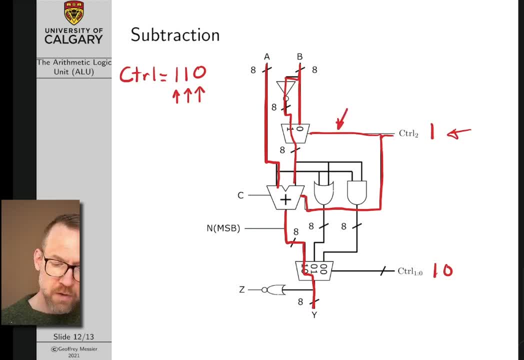 So this part of the control two line does bitwise inversion or finds the bitwise complement. So this part of the control two line does a bitwise inversion of b. However, this part adds one to the bitwise complement of b And those two operations together negate b. 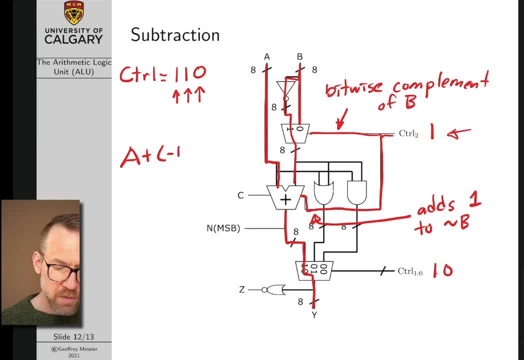 And as a result, we get a added to the negative value of b, or in other words a minus b, And so that's how subtraction is implemented. Just a few, or just another quick word about these, about our flag outputs. 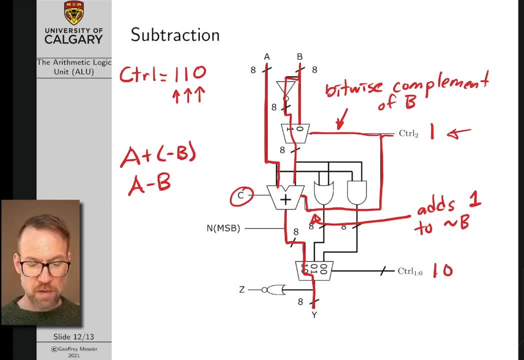 So I talked about the carry out. So that's just the carry out bit of the most significant single bit addition in our ripple adder. The negative flag is just the most significant bit of the output of our adder. Remember our sign bit is the most significant bit. 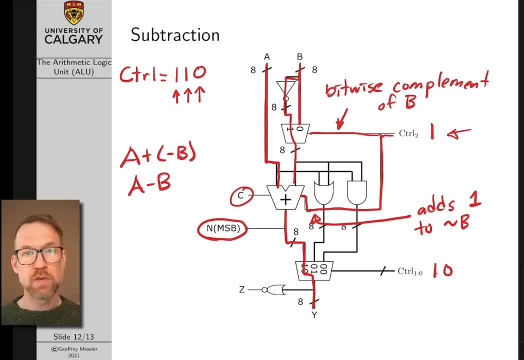 in two's complement. If it's equal to zero, it's a positive number, If it's equal to one, it's a negative number. So we just have to pull off that most significant bit And that gives us our negative flag. 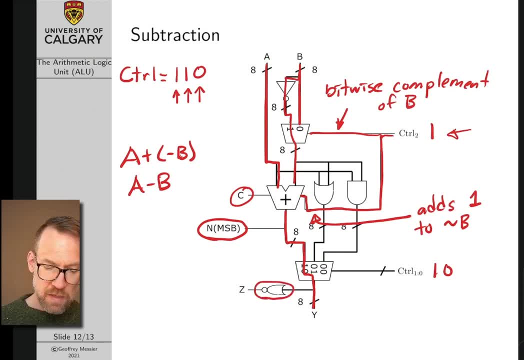 And finally, the zero flag is the NOR operation performed on all three of our- or sorry, all eight of our outputs. So if all eight of our outputs are equal to zero, we have. our zero flag is equal to zero. So if all eight of our outputs are equal to zero, 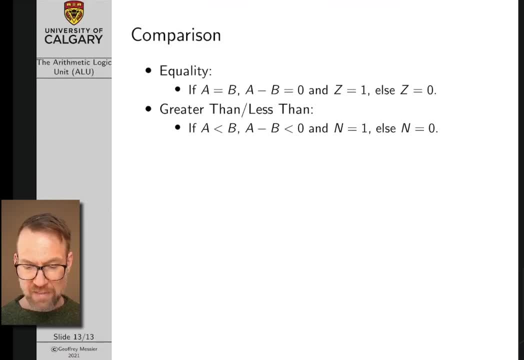 we have, our negative flag is equal to one. Otherwise, the zero flag is equal to zero And, just like I said at the start of the lecture, we can use the zero flag and the negative flag to test for equality and greater than or less than.